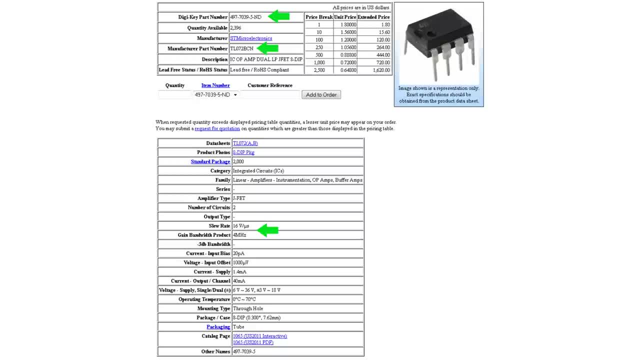 14 volts per microsecond. The op-amp you use will have to have similar specs or better, so that it can operate as an oscillator well into the megahertz range. It will also have to be able to handle at least 9 volts. 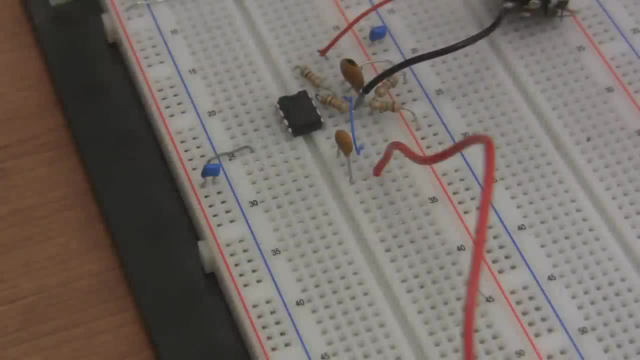 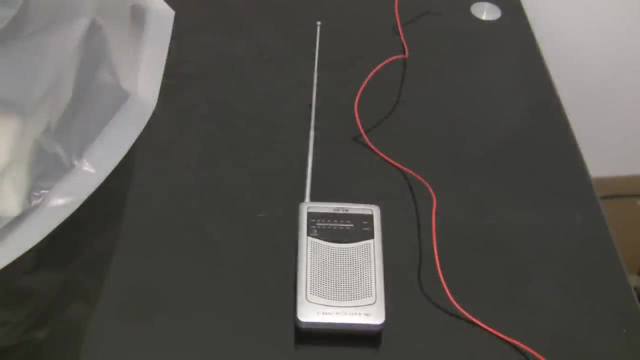 OK, so you've got your oscillator. Now, if you add a long piece of wire to the output of the oscillator- at least a meter long- some of the energy from the oscillations will be converted to radio waves and you'll have a very crude radio transmission. 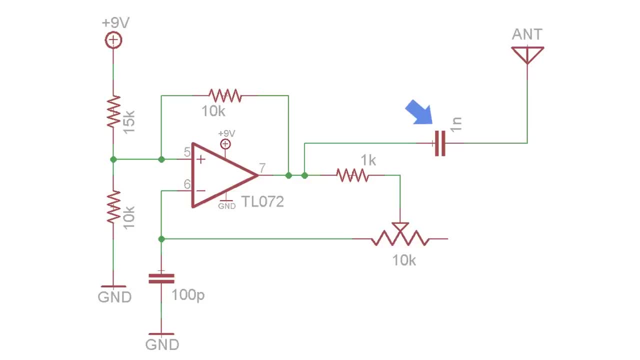 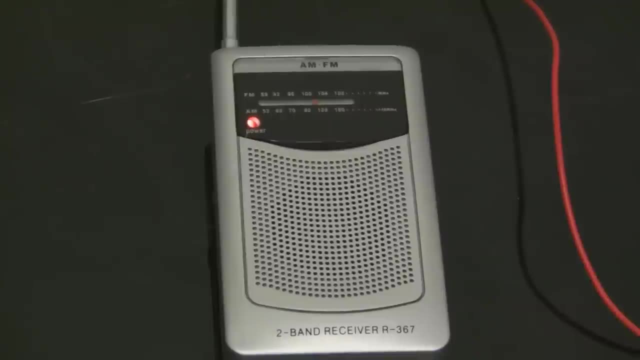 By the way, you always want a capacitor before your antenna to protect your circuit and block any DC voltages the antenna may accidentally touch. Now I'm almost ready to show you a simple telegraph, but first you'll have to bear with me. 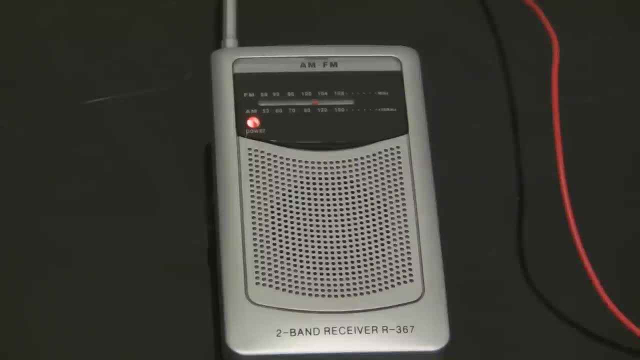 I live near a broadcasting tower and there's no way for me to get total radio silence on this cheap little radio. So if you hear a boring news broadcast, just pretend that it's white noise from an empty station. Right now the AM radio spectrum around me seems quietest, around 900 kilohertz. 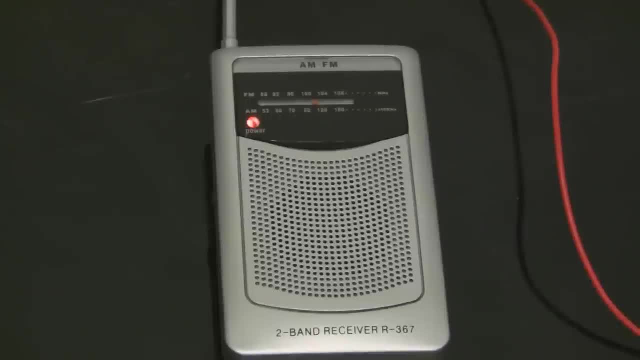 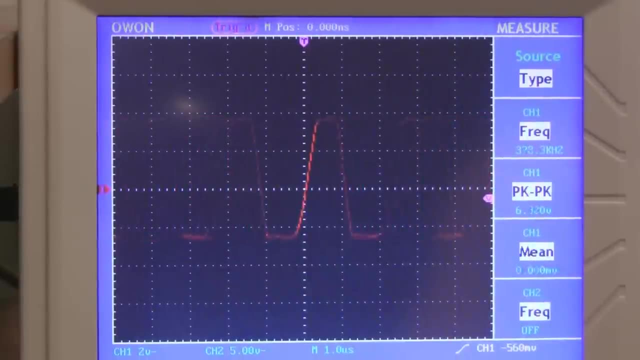 So let's see what happens when I adjust the frequency of my oscillator to around 900 kilohertz. At 950 kilohertz you'll notice that the receiver goes totally silent. That's because it's detecting the radio waves that I'm transmitting instead of picking up. 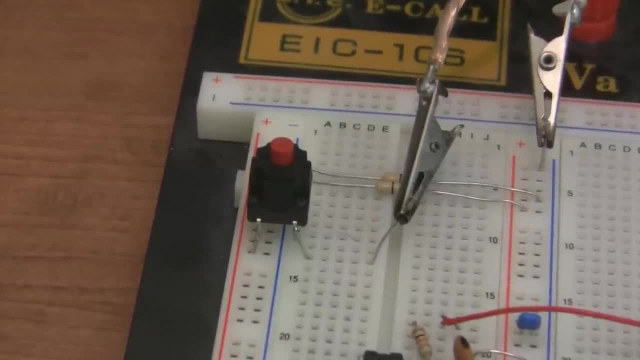 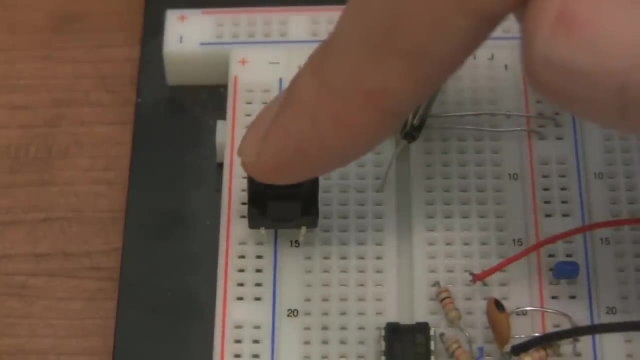 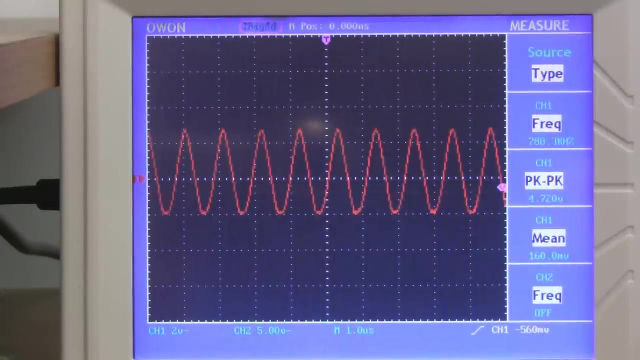 random noise. Now this is where the fun starts. If I put a switch on the 9 volt supply line, I can turn the oscillator on and off, which will cause the waves to be transmitted in little pulses. So now I can tap things out in Morse code and somebody tuned in can tell me that I'm 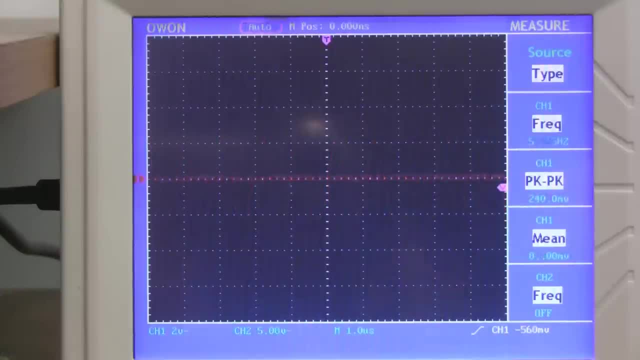 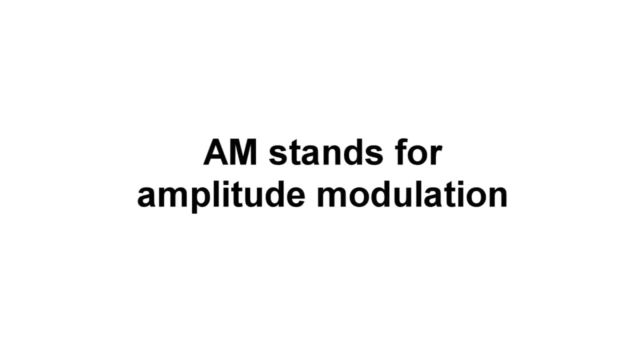 listening. The modern term for this is on-off keying, because the only thing I'm doing is turning the oscillator on and off and sending out radio waves in little pulses. OK, now what is AM? AM is amplitude modulation. I should probably explain what modulation is. 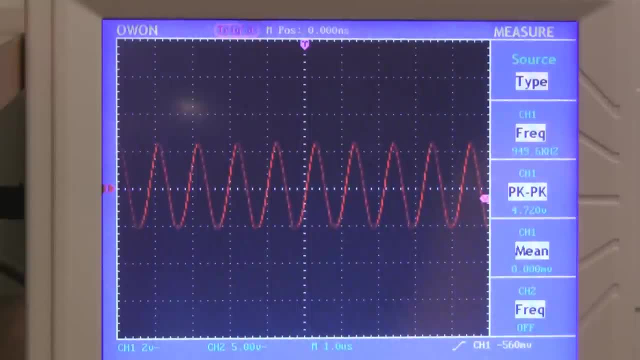 You know how. we started out by transmitting a wave of 950 kilohertz and the receiver detected it. That wave is called the carrier wave and it's typically of a high frequency, anywhere from 100 kilohertz to 10 gigahertz and beyond. 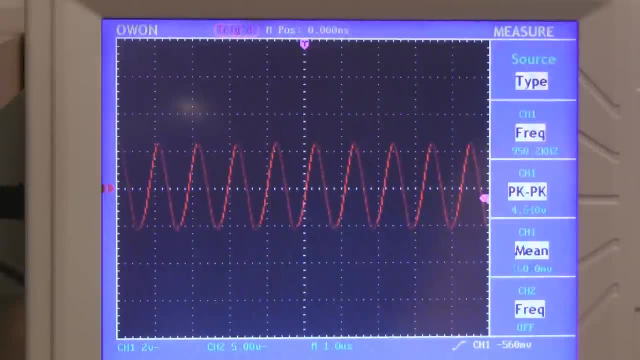 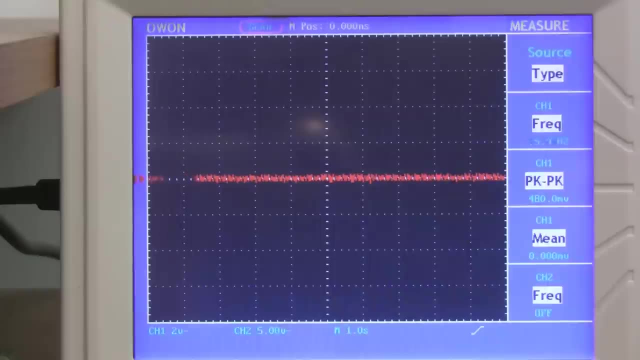 That carrier wave on its own isn't really useful for any kind of data transmission. All we got was constant radio silence. But when I started turning the oscillator on and off by hand, I was able to send out messages in Morse code. 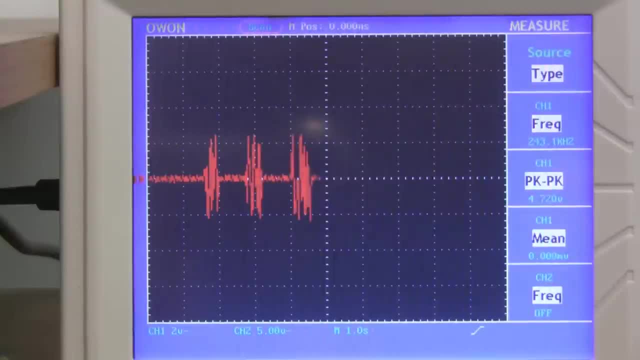 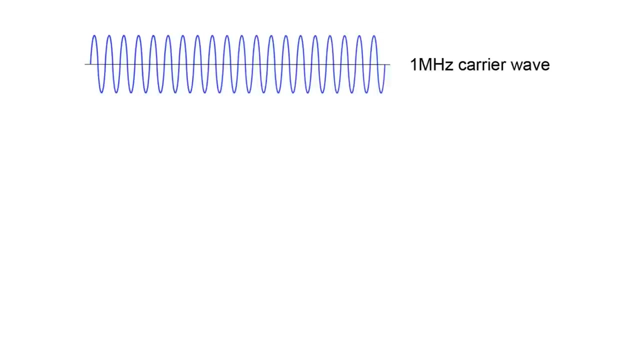 The process of manipulating the carrier wave to carry useful data is called modulation, And there are many, many ways you can manipulate a carrier wave, but one of the easiest to understand is amplitude modulation. AM allows you to send an analog signal, like your voice, over long distances. 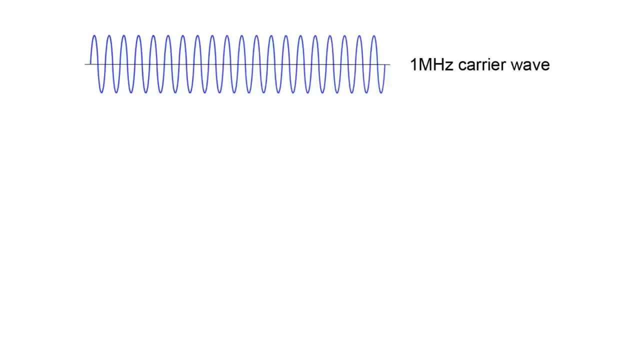 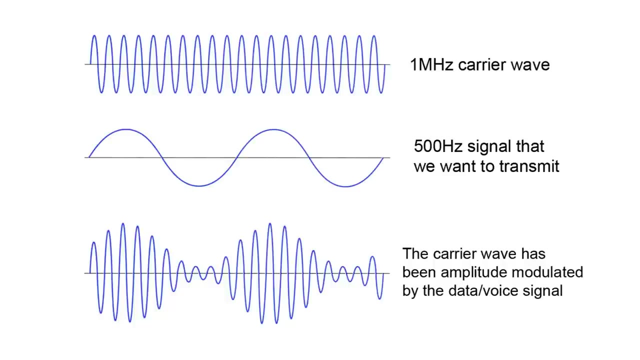 It works like this. Here's your carrier wave, a continuous wave of, say, 1 megahertz. Here's a lower frequency voice signal, let's say a sine wave of 500 hertz for now. Now, if I create a circuit that uses the amplitude of the voice signal to vary the amplitude, 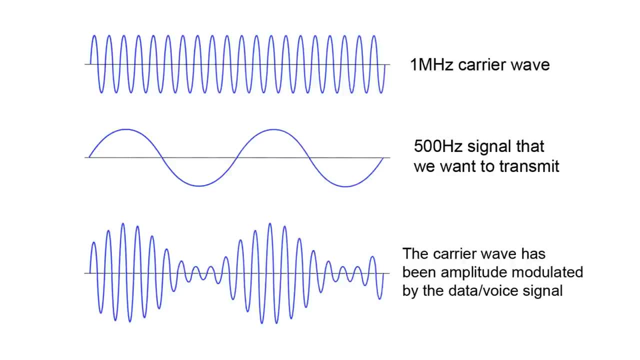 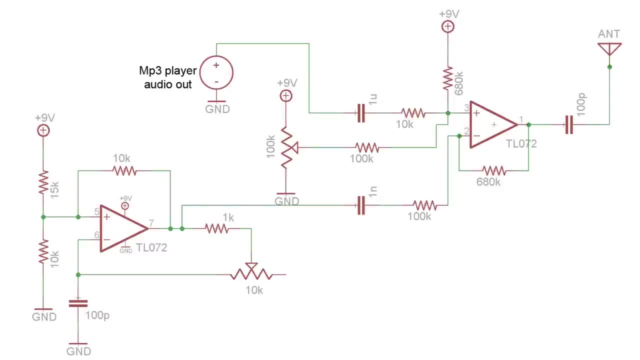 of the carrier wave. I will have amplitude modulated the carrier wave And, more realistically, this is what it would look like with voice or music. So let's take a look at a circuit that can do this. The first half is the oscillator that you've already seen. 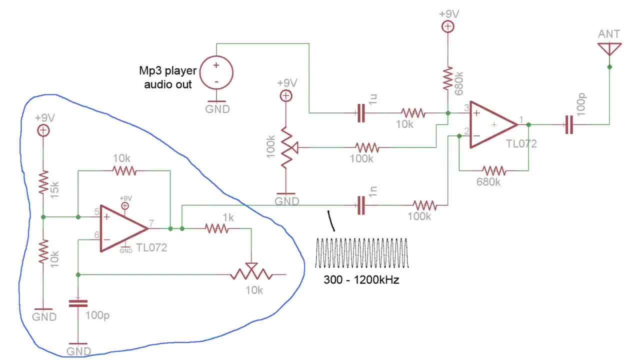 It generates the carrier wave, which is a continuous high frequency sinusoid. Over here we have a high pass filter to remove the DC offset from the oscillator's output. The high resistance of 100k also helps to isolate the oscillator from the modulator. 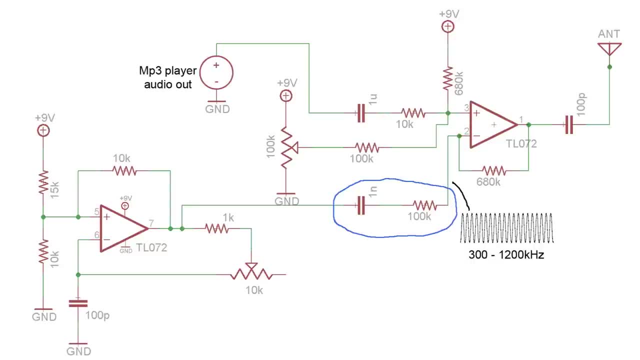 so that the modulator doesn't mess up the generation of a frequency stable carrier wave Over. here we have another high pass filter to ensure that we're only getting AC audio from our mp3 player or other audio source. Finally, the op amp circuit on the right will take the audio signal from my mp3 player and 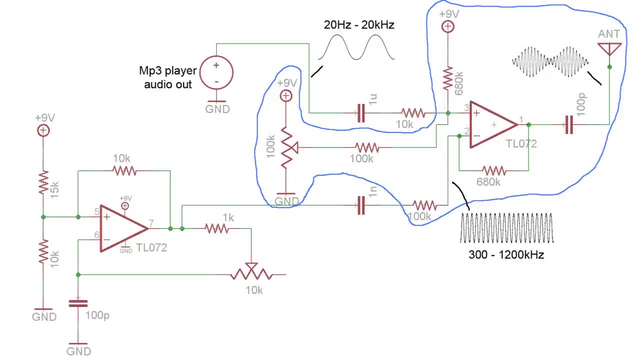 use it to dynamically adjust the amplitude of the carrier wave. The potentiometer on the left controls the amount of modulated audio and the potentiometer on the right controls the amplitude of the carrier wave. The potentiometer on the right controls the amount of modulation, and it also provides 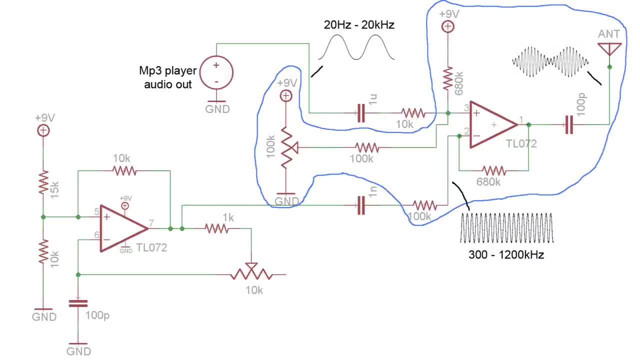 a DC operating point for the circuit to work at, And once we have that amplitude modulated signal, you can hook it up to an antenna and some of the energy will radiate out in the form of radio waves. Okay, let's hook up the mp3 player and start modulating the carrier wave. 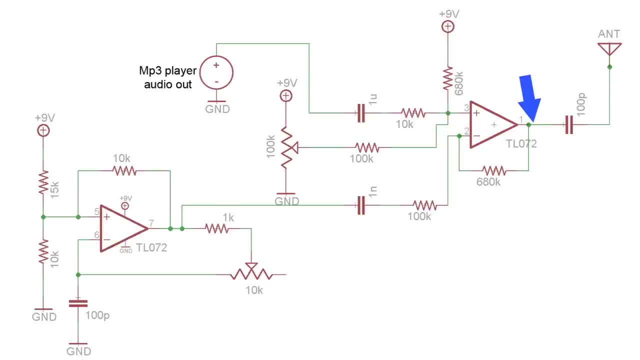 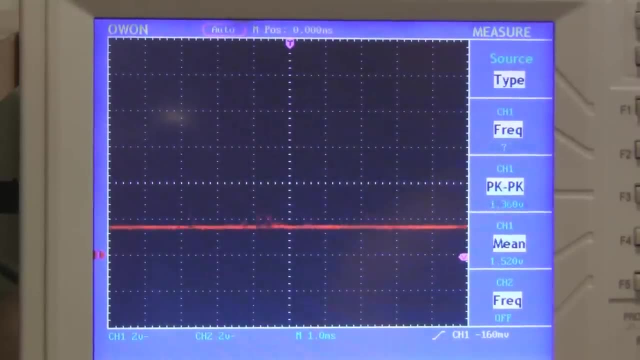 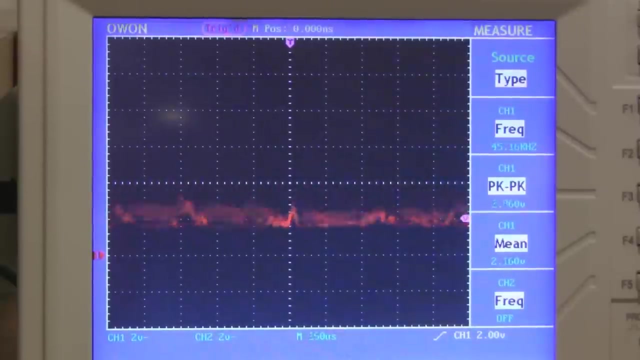 My oscilloscope will be displaying the voltage right at the modulator's output before the antenna. And there you have it: a simple AM radio transmitter. Also, if we zoom in on the amplitude modulated signal, we can see that it's still based on. 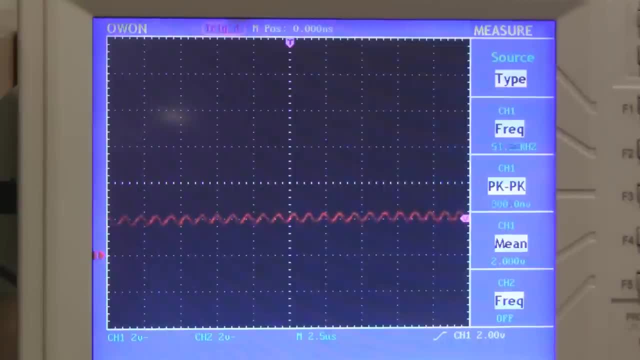 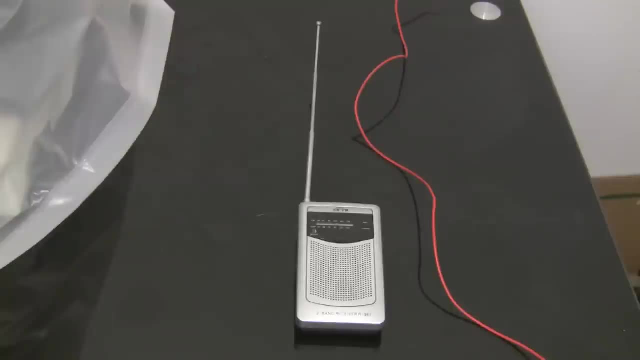 the 950kHz carrier wave. This is a very low powered, unoptimized design, so don't worry about any legal issues. it's only going to have a range of a couple of centimeters. If you want a little bit more range, add a 220uF modulator. 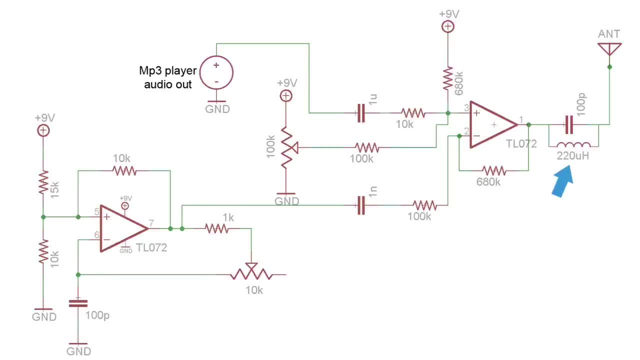 And that's it for this video. I hope you enjoyed it. Thanks for watching. I'll see you in the next video. Bye, bye. Finally, I'd like to thank Stefan0719 for the circuit designs used in this video. Check out his channel for more great circuits. 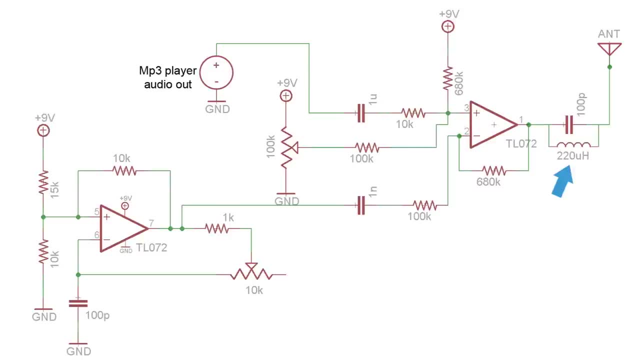 I'll do a video on LC filters and resonance in the future. Finally, I'd like to thank Stefan0719 for the circuit designs used in this video. Check out his channel for more great circuits. I'll see you in the next video.